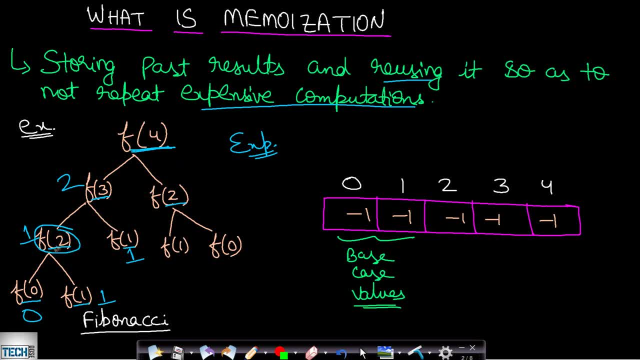 Since I have drawn a smaller structure, it is not much visible, but you can see that F of 2 and F of 2 is repeating here. Okay, and if your tree is much larger, then you will find much more repeating sub problems. So the second time you don't need to call this F of 1 and F of 0. When you have already. 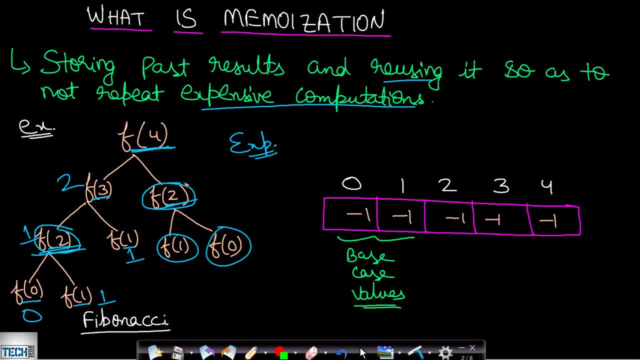 computed this F of 2, then you can simply use that value and you can return from this part. Okay, so this will reduce the number of function calls in case of recursion and hence it will optimize the solution. This is known as memoization, that is, storing the already computed value, like here you had no. 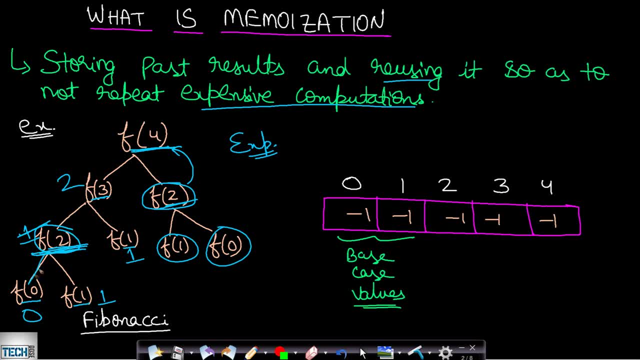 knowledge of what the F of 2 value is. and so you went through with the recursion and when you returned, then you were storing the values in your table. Okay, so let's say we are storing in a table, you can use anything, you can use a map or a table or anything. So we were storing in the table and 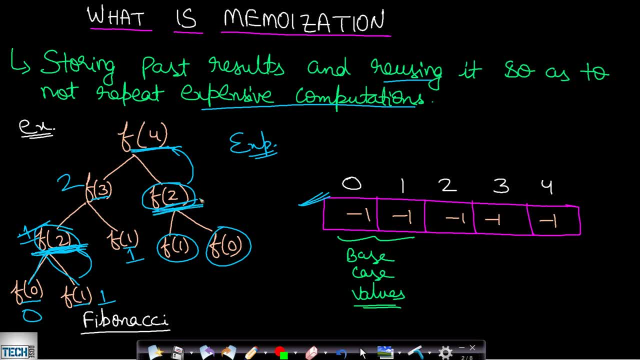 then, once we have stored all the values now, if we are encountering the same problem, then we will use the table and return the value. in that way, we will be reducing the time complexity. Now, when we are using the table, then we will be having certain base cases here: F of 0, F of 1 and having values 0. 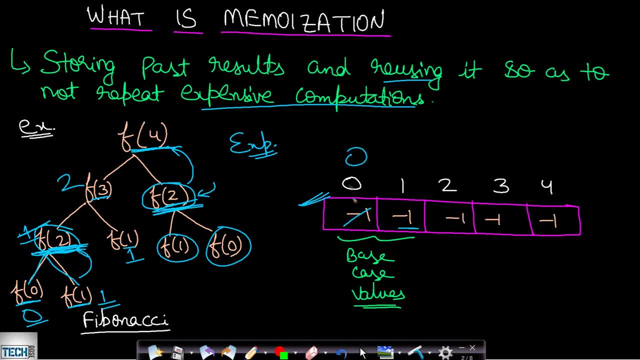 and 1. So initially F of 0 we will be having values, F of 1 will be having value 1 and rest of the table will be marked as minus 1, indicating that the values have not been found yet. so if let's say you 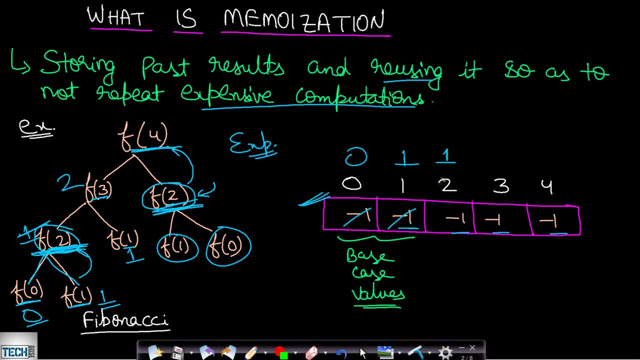 have found the value of F of 2.. And you Have here one, okay, and again you are encountering this f of two. then you will look at this table value and see that it is not minus one and it is one. so since it is a positive number, it is already. 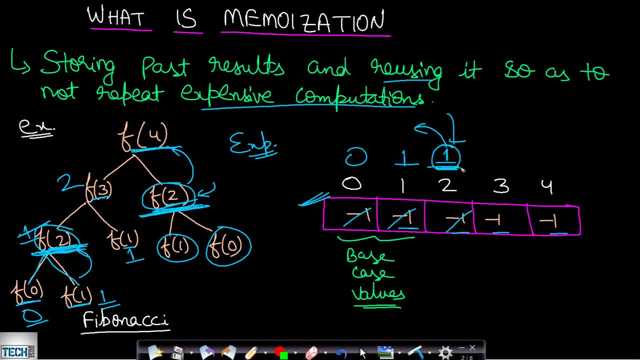 calculated and therefore, you will return this value. okay, you don't need to calculate what the values f of two is so like that. you can implement a table or a map or any other data structure in order to store all the values, and this will help you reduce the time complexity. okay, so this is. 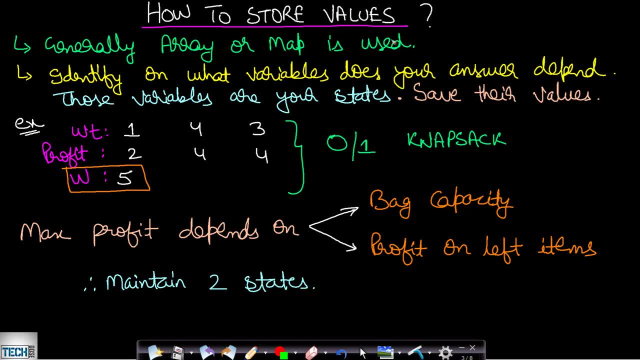 the entire idea of mememization. now, how to store the values. generally, we use array or map in order to store the values, but we need to identify on what variables does your answer depend? those variables are your states and we need to save their values. so let's say we are taking 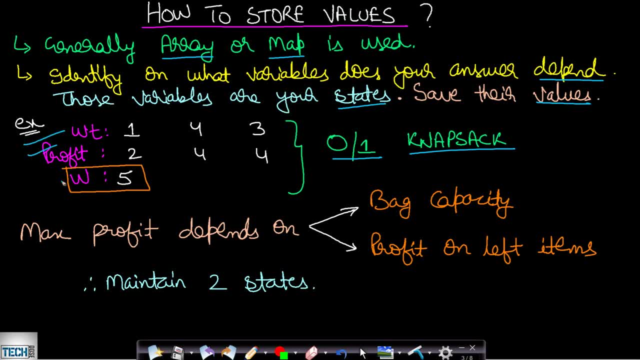 this example of 0, 1 next. so we are given weight, profit and the capacity of the bag. now on what parameters will your maximum profit depend if you are given a bag having certain capacities will be fixed now on what we are taking. this, mesela, look at number 5, which I 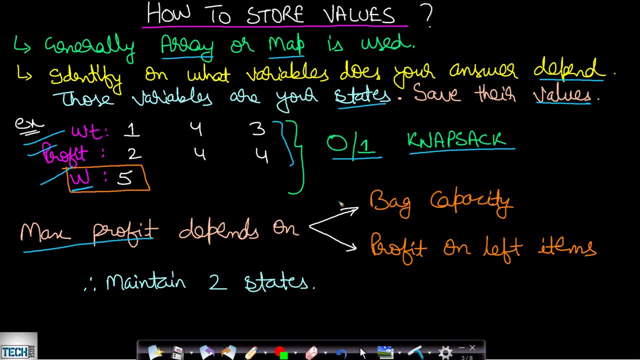 capacity and certain number of items, then obviously the maximum profit will depend on what is the capacity of the bag, because if the capacity of the bag is more, then obviously you will be getting at least greater than equals profit. okay, and your profit also depends on your items. so whatever number of items you are having as options to select, and what is the capacity of 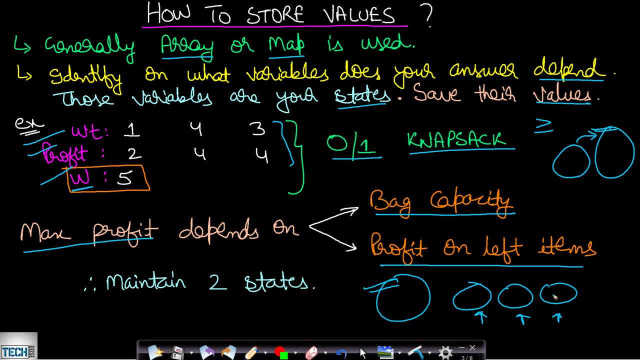 the bag. on these two factors depends the maximum profit. okay, so we need to maintain two states, because our maximum profit depends on two variables, that is, two states. so this you need to consider for each and every problem on dp which you are solving by memoization, if you are able to solve. 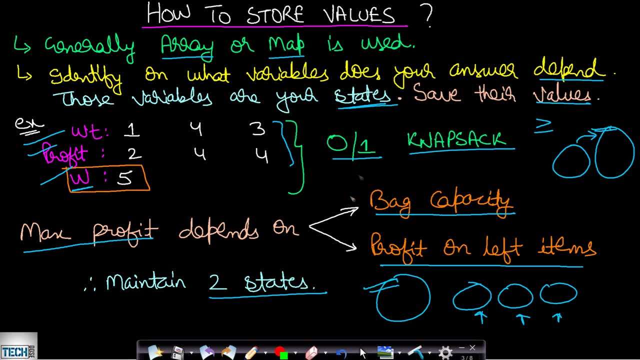 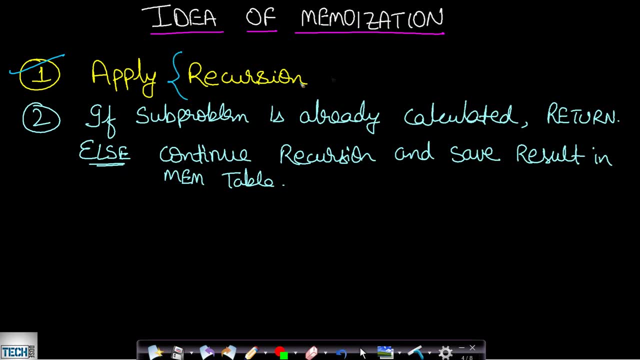 by recursion, then obviously you will be knowing about the states on which it depends. now let us see the idea of memoization. it is based on a simple idea of smart recursion. so this is recursion plus and minus. so this is recursion plus and minus. so this is recursion plus and minus. 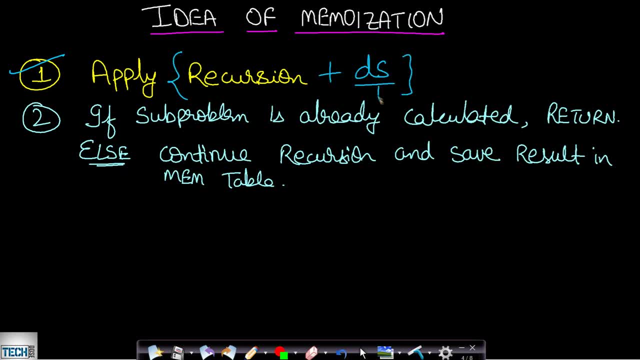 using certain data structure in order to store your already computed values, and that is nothing but smart recursion. this is also known as dynamic programming, because you are already remembering the computed results. so remembering the past results and using it again is known as dynamic programming. now, if the sub problem is already calculated, then we will be returning by using 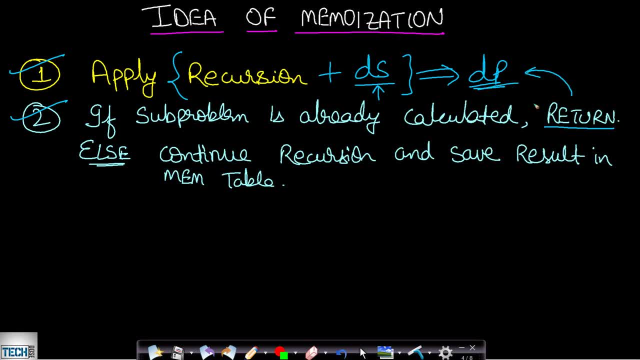 the table which we will be filling. otherwise, if it is not already calculated, then we will continue our recursion flow and when we return from our recursion call then we will be saving the result in our dp table and then we will be using it if we encounter that. 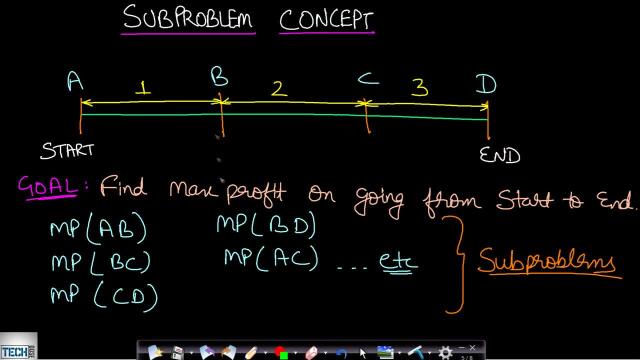 sub problem again. okay, so this is the idea of memoization. now, what is a sub problem? if you are confused about sub problem, then what it really means. let us say that there is a problem given where we need to start from some starting- point a- and we need to reach to the ending point. 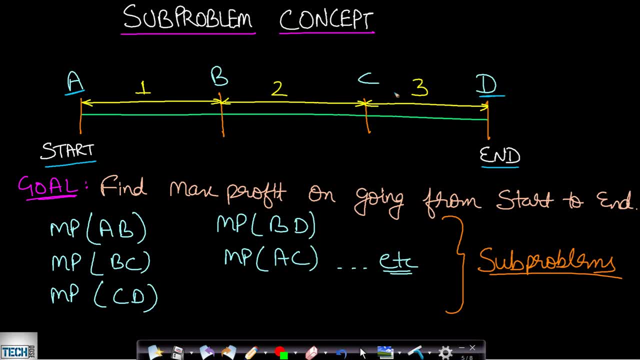 d and we need to maximize our profit. okay, so in this case you can say that the problem states that you want to find maximum profit in order to start from a and reach to d. okay, now this problem can be further broken down into sub problem. let's say, if you break down, then the maximum profit. 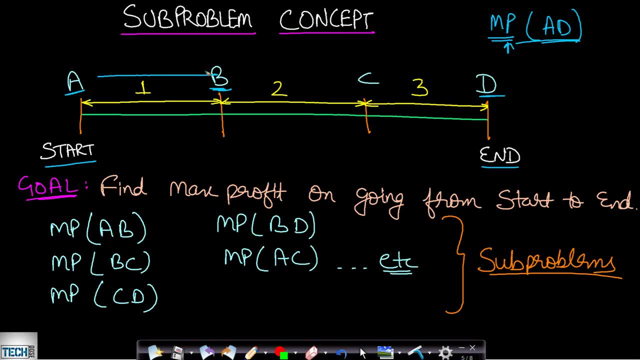 in order to reach to this, b from a will be something. let's say it's one. now, the maximum profit from b to c is 2 and maximum profit from c to d is 3. so since you know in segments what is the maximum profit from a to b, b to c and c to d, you can combine them all and you can find the. 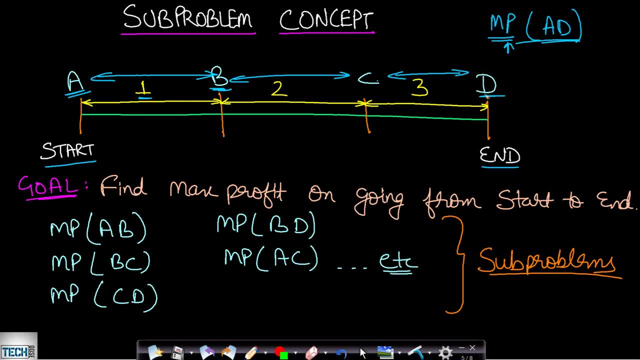 maximum profit from a to d. okay, so this is one case. this is a very simple case and in this case, a to d is our entire problem and since we have divided the problem into segments, that is, into sub problems, you can find the maximum profit from b to c and c to d, and you can find the maximum profit. 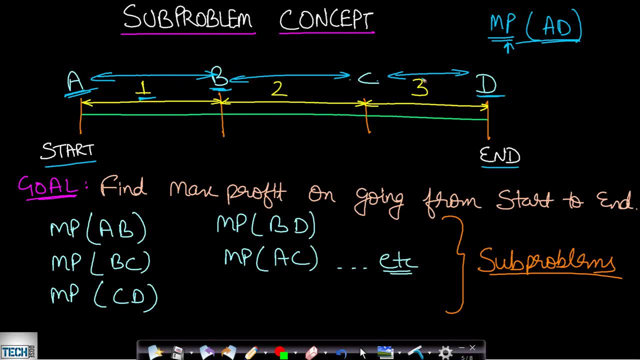 okay, so this is one case. this is a very simple case and in this case, a to d is our entire problem. therefore, we can combine the solution of the sub problems and we can find the solution for the bigger problem. so in this case, you can say that the maximum profit of 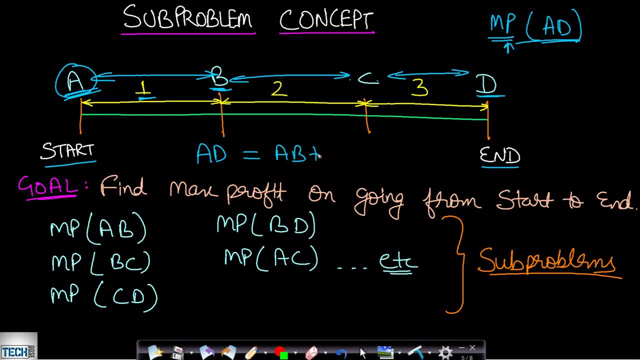 a to d will be equals to maximum profit of a to b plus b to c plus c to d. otherwise you can also break it in certain other way, like: the maximum profit from a to d can be written as maximum profit from a to c and from c to d, okay. or you can have other combinations, like from a to b. 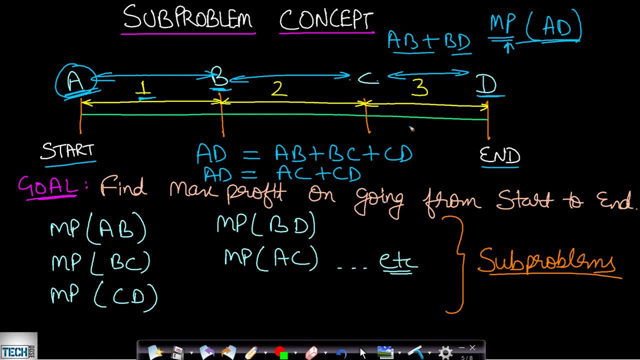 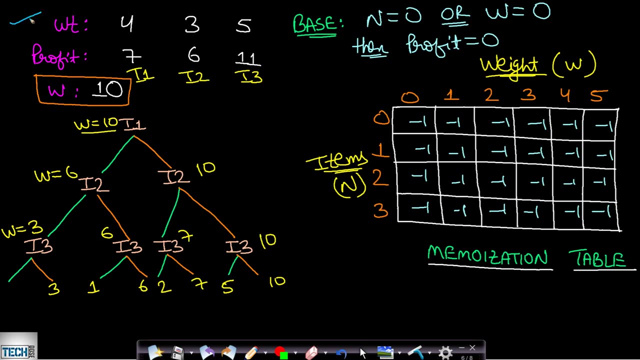 and from b to d any other combination. okay, so these all smaller parts which will be used in order to form the solution for a bigger problem is known as the sub problem. i hope you got the understanding here. so once you know about sub problem, let's see this zero one knapsack problem. 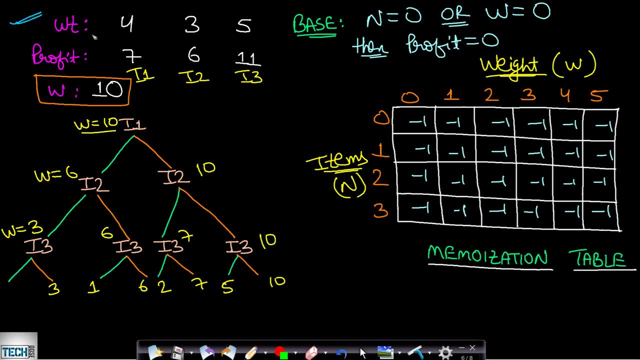 and how it is solved by using memoization. in this case, i have taken certain items- there are three- number of items, along with its associated weight and profit, and we are given a bag having capital capacity as 10. now, as i had already explained in my previous video, which is a prerequisite- 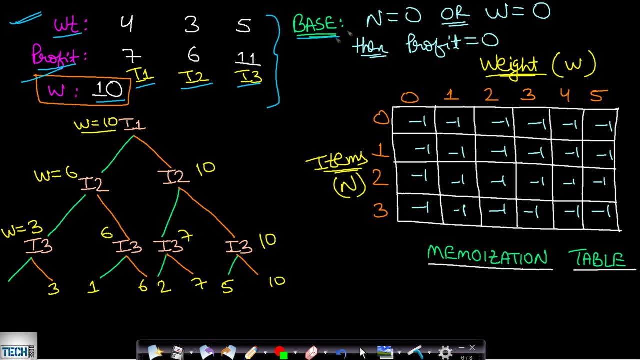 for watching this video, obviously so. in this case, the base case was: if you have no items, then you cannot gain any profit. otherwise, if you have no capacity in the bag, then you cannot gain any profit. in either of these two cases you won't have any profit, and so you will be just. 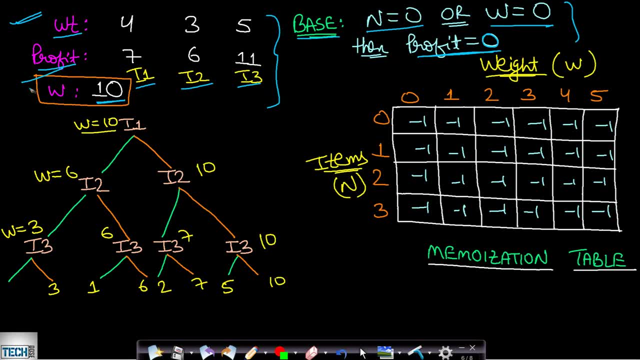 returning profit as zero. in all other cases where you have capacity and you have items, you will try to accommodate effects in terms of that previous video as much as possible, but you can learn other Villarrealization and understanding if you want to strengthen your value chain. the 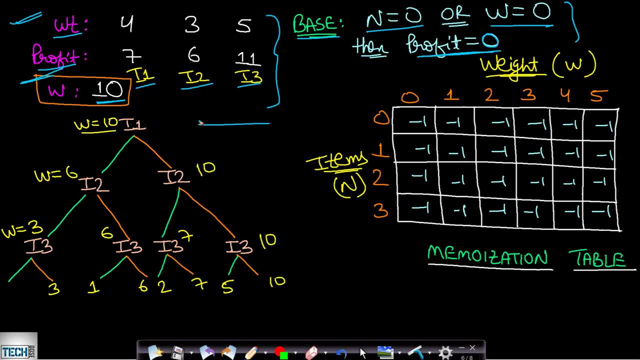 added items into your bag. okay, so this first level will be indicating item one. second level, item two, third level, item three, and how it is done. let's see so, initially you will be at this item one. now, when you are at this one, you can either include it or exclude it. so this green line, 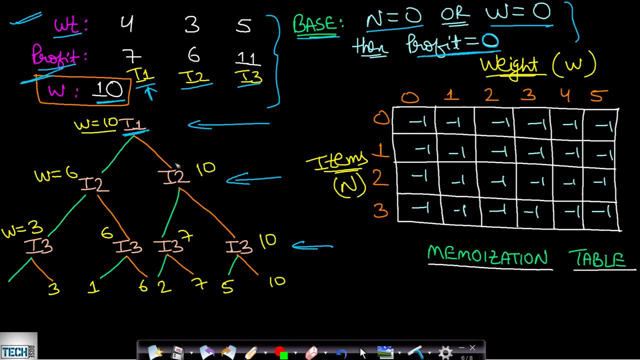 indicates that the parent node is included and red line indicates that the parent node is excluded. so this line i1- i2 is indicating that i1 is included. okay, the green line. so if you have initial capacity as weight equals to 10 and your item 1 is included, which is having weight equals, 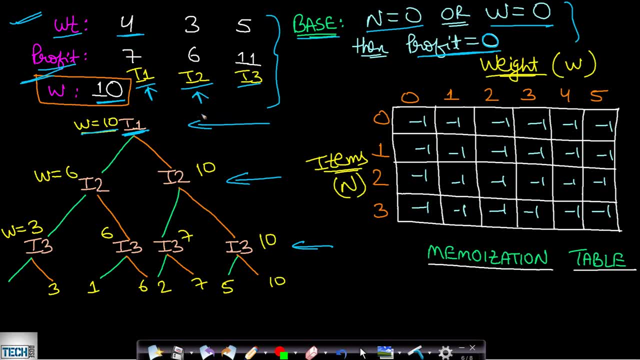 to 4, then when you reach to this item 2, then you will be having capacity equals to 6, because item 1, having weight 4, was included. okay, and now at item 2 you have two options and let's say you select this item 2, then weight 3. 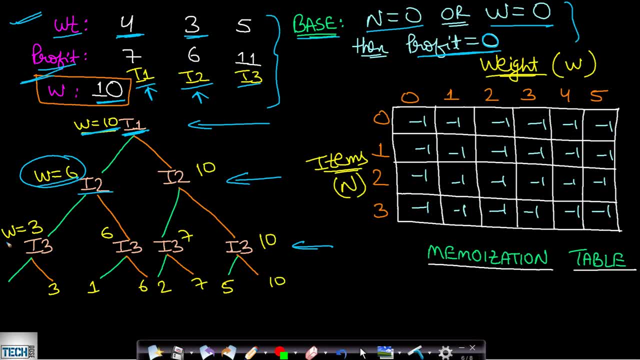 3 will be added into your bag and so the capacity will reduce. so capacity will be 3 now, and when you are at item 3, you have capacity 3 and the weight of item 3 is 5. so you have just one option: you have to exclude this item 3. okay, you cannot include it like that. you will have to perform all. 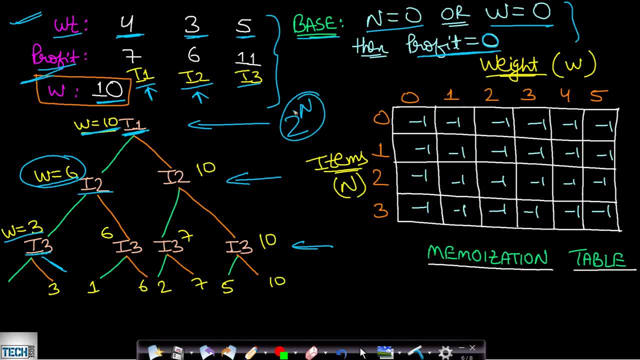 possibilities, and this will take exponential time, as i had explained in my previous video using recursion. now our goal is to optimize it. our goal is to apply smart recursion, that is, we need to memoize it. now, how do we store the result? as i had already explained, there are two states on which 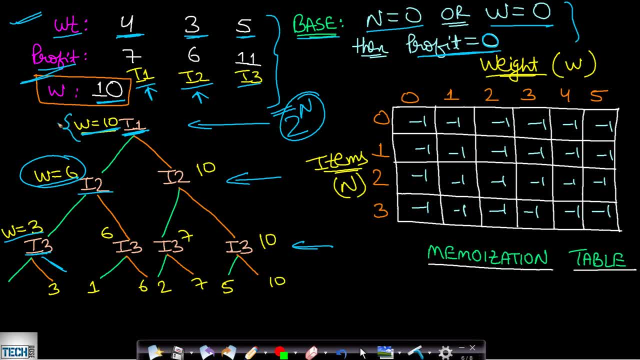 your maximum profit will depend. it will depend on the capacity of the bag, which is w, and also on the number of items. so we can create a table where the row number will indicate the number of items and the column number will indicate the capacity left in the bag. okay, so let's say you have a. 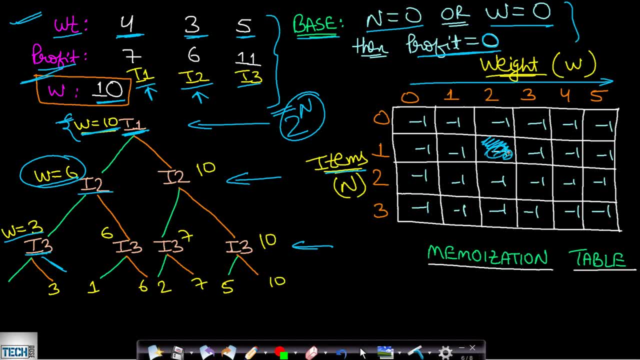 problem like this one. this is a sub problem, okay, you. so this sub problem is indicating that when you have item one and when your capacity of the bag is two, then what will be the maximum profit? okay now. this sub problem is indicating that when you have all the three items and your capacity of the bag is three, then what will be the maximum profit. 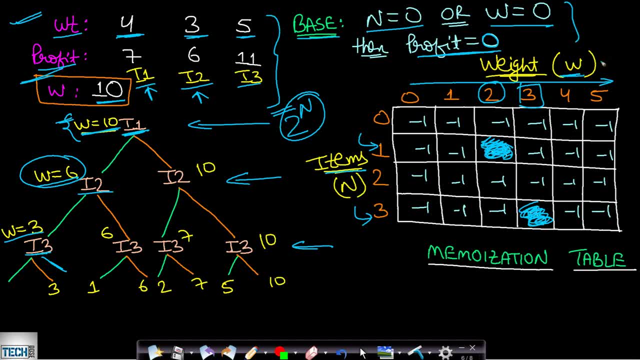 okay. so in this case i am assuming that weight available is equal to five only. so in this case, let's say, if you have all these three items and your capacity of the bag is three, then obviously you will be only able to include this item because this item is having higher. 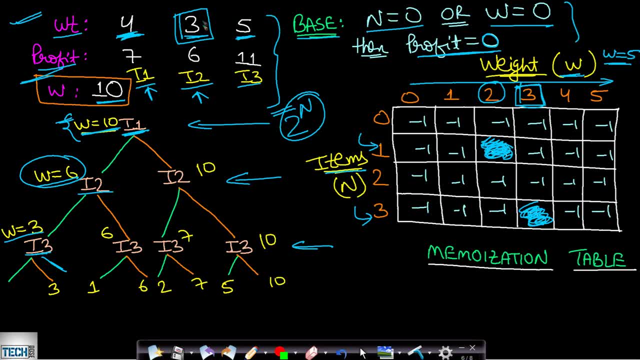 weight four and this is higher weight five. so since we are including this weight, our profit will be six. so this sub problem, which will be dp, or let's call it memoization- memoization at three and three- will be equals to six, because the maximum profit will be six. 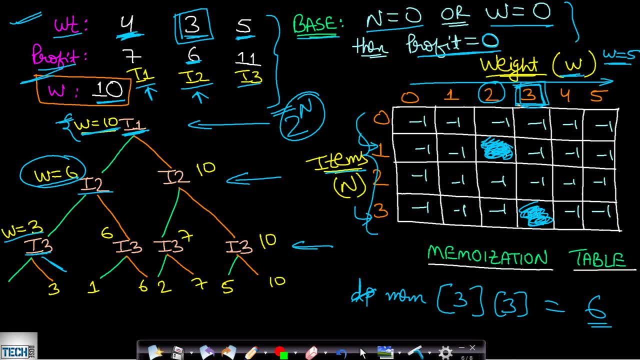 when you are having all the three items and you are having capacity of the bag, as three will be equals to six and the entire problem will be this last row and last column, this last cell. okay, so this will be indicating your entire problem. this is indicating that. 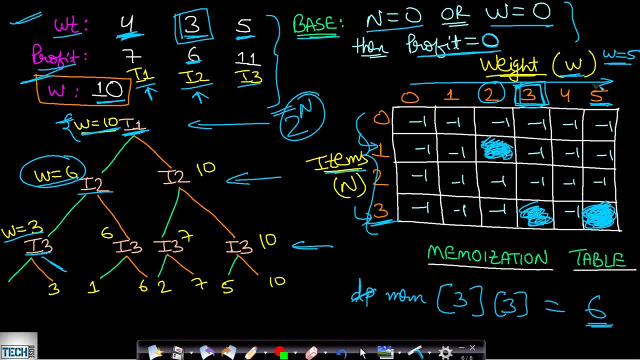 when you have all the three items and you have the entire bag empty, which is of size five, then what will be the maximum profit? and this was our entire problem, okay, so if you have all the three and your capacity of the bag is five, then obviously you will get maximum profit on. 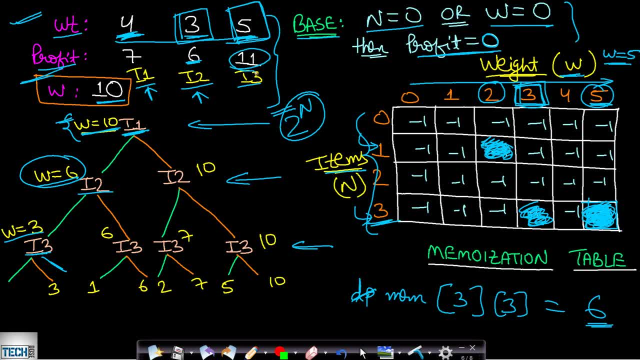 including this part. okay, this third item, which will be profit, equals to 11.. so memoization at 3 and at 5 will be equals to 11.. this will indicate the maximum profit when you have all the three items and you have capacity of the bag as 5.. so this is how we can represent a sub problem. 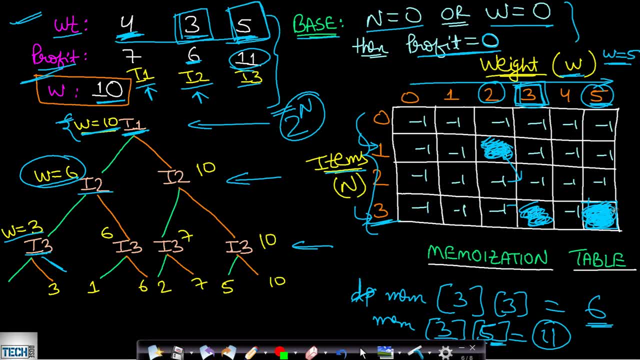 and this is how, by solving and combining all the sub problems, we can solve the bigger sub problem. so this last cell is the bigger sub problem, which is the entire problem itself. so the only thing is that we should know about the base cases and we should be able to write. 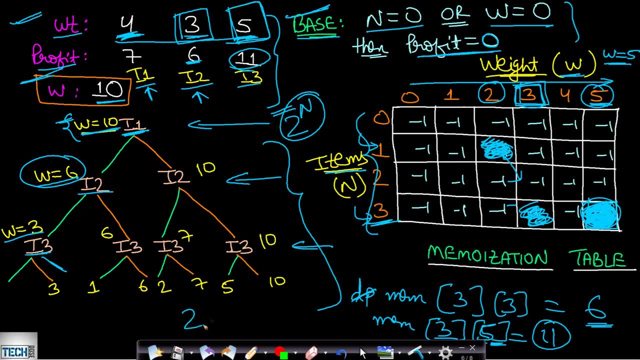 the recursive code. once you write the recursive code, you can add two lines into this recursive code in order to get this memoization code. okay, and you need to include a data structure, so for that you need to identify the states. this will come with practice, okay, so this is the code. 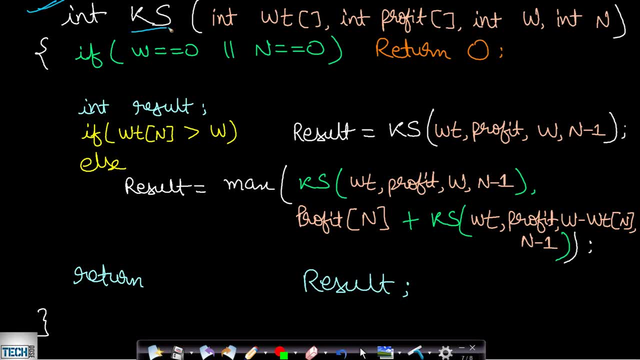 for the recursion which i had shown in my previous video. so this is the napsack 01 napsack. here our input was weight profit, this was our capacity of the bag and this was our current item which we were processing. so initially we will be having the 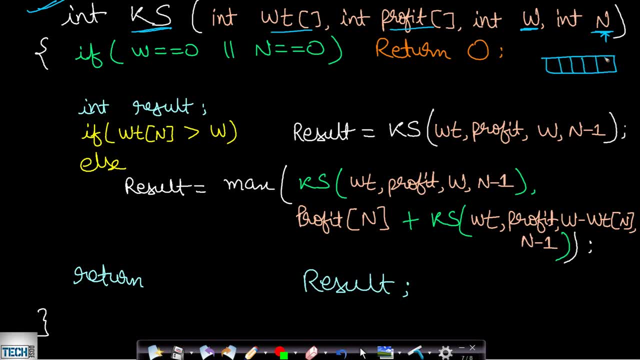 entire array, okay, entire array of items, and initially we will be having all the n items, so this will be n items. now, once we use this item, then we will be having n minus one items. so we will be calling from right to left, okay, and we will be. 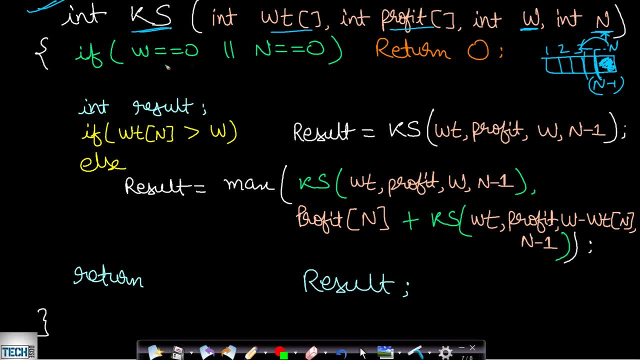 getting the class weights from left to right. so this is the main problem, part of the problem, and also the size of the array. so in this case- this you must have understood from the previous video- this is our base case, when you have no items or you have no space left in your bag. 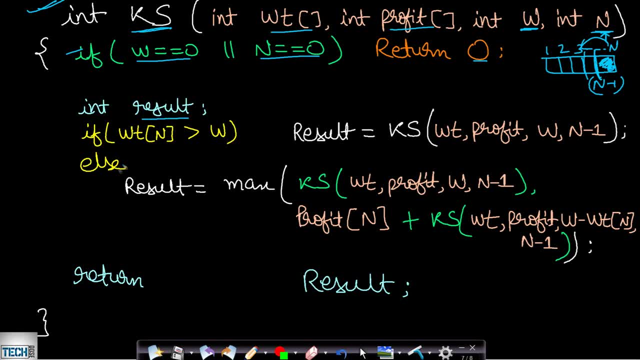 you will have to return zero as profit. this is our result, which will be storing the result of the two choices. i had already explained that if the item weight is greater than the capacity of the bag, then obviously you cannot fit it into the bag, and so your only option will be to exclude this item, and you can remove this item as well. 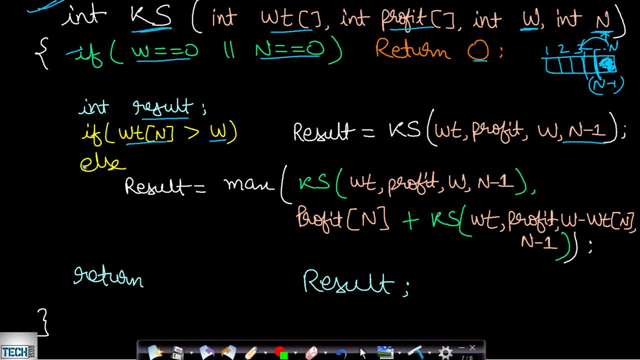 and you will have to record for the rest of the items and if the item weight is less than equals to the capacity of the bag, so you can include it or you can exclude it, so we will take the maximum of the two choices. okay, so this was our recursive program. now how do 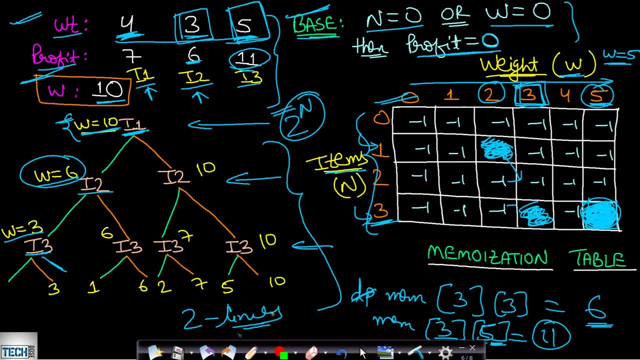 we apply memoization here. so, as i had already explained, you will have to take this table, however you take. okay, you can also take a single dimensional table using a string as your key map, or you can take a map, but for just for simplicity, i am explaining here that. 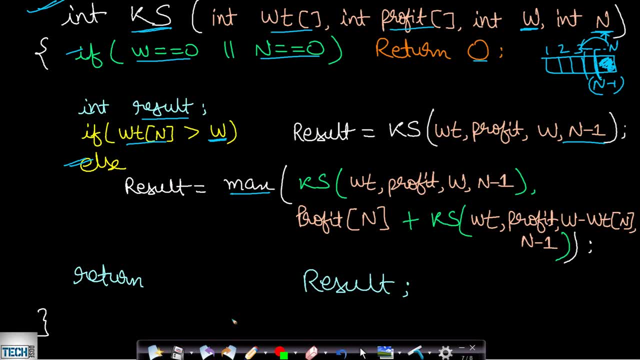 you can take a 2d array now. once you have taken that, then you need to add just two lines, as i had said. so the first line will be for storing the result. the result is calculated and that should be stored into your map- okay, into your array. so initially it was minus. 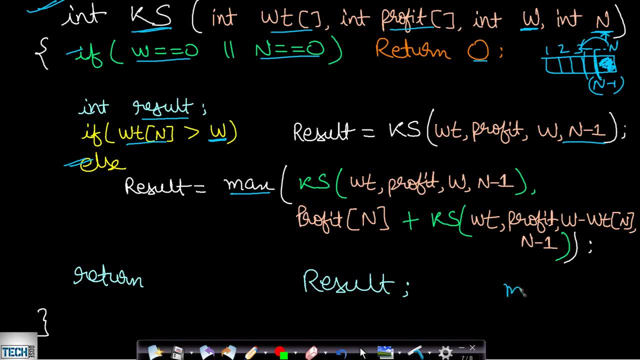 one all over. so how do you store it? let's say your array name is memoization mem, and here you should have your name and your array name. you should have your name and your array. that is a two-dimensional array. the first dimension is for the capacity of the bag. 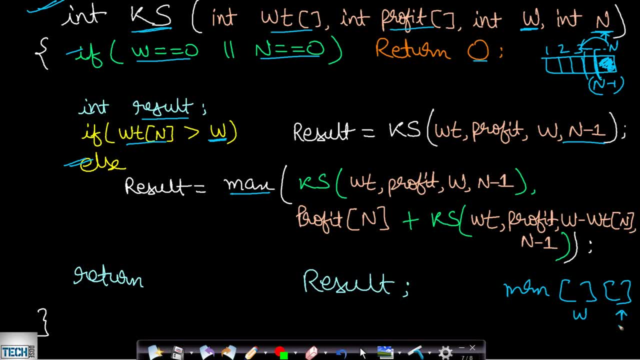 which is the current capacity, and this is the item. okay, that is a number of items. so here what you can do is you can store the result as mem at w and that n that will be equals to result. and how i am storing it, because you have found the maximum profit here and stored it in. 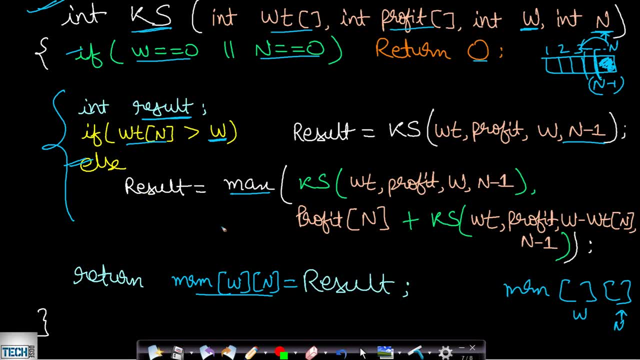 result now, since you are calculating it, so you need to update your dp table. okay, this is your memoization table. that is why we are storing, for this sub problem, the result value. now, how do we optimize this entire approach? well, we have updated our dp table, which is our memoization table. 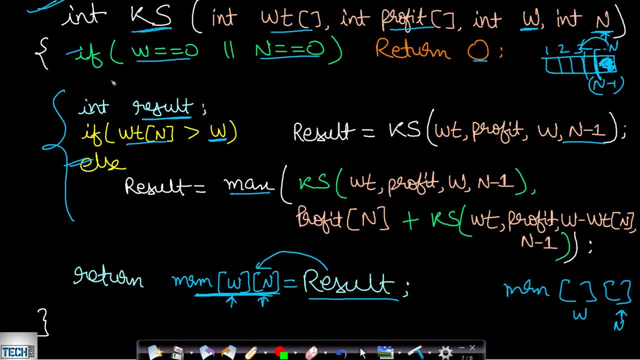 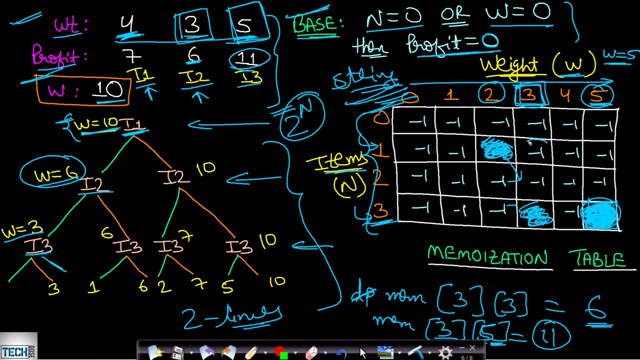 so we will have to look up initially so that if the value is already filled then we will simply return without doing this processing part. so we need to add here: if memoization at w, which is the capacity of the bag, and that n, which is the number of items, current number of items, is not equals to minus one, if the value that is a sub. 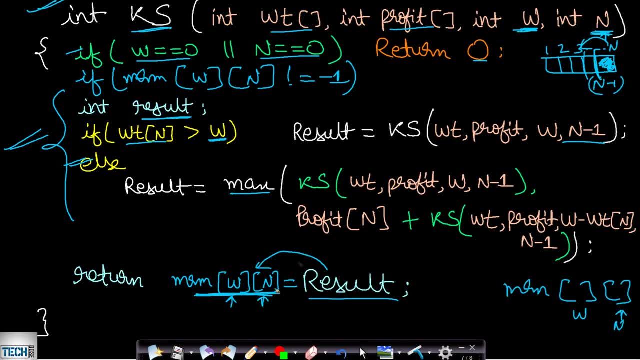 problem is not equals to minus one, then obviously it has been calculated and so you can return whatever the value is at memoization, at w and at n. okay, so this is used as lookup. so here you are just checking if the sub problem was already calculated, and in the last line you 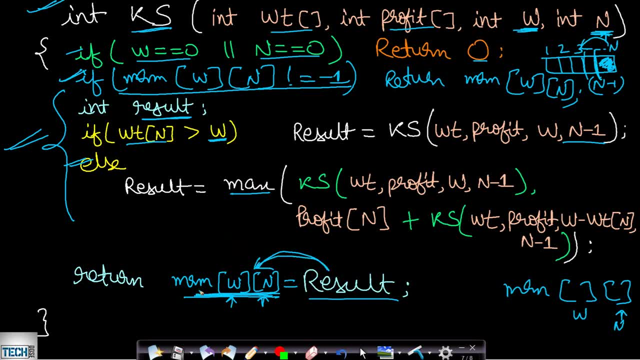 are storing the result, which is the maximum profit, into your sub problem, which is at wth row and nth column. okay, so this is used for updation and this is used for lookup. that is your return. so these two operations will together improve your time, complexity and what will be that.